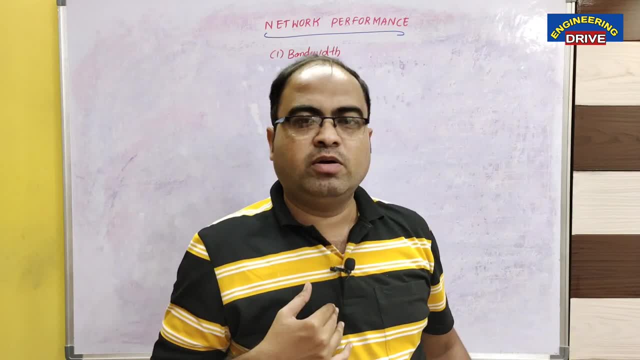 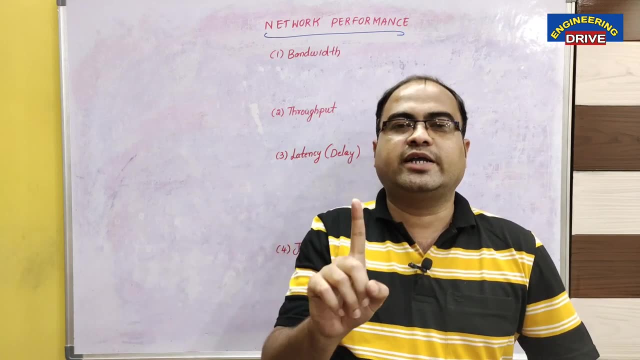 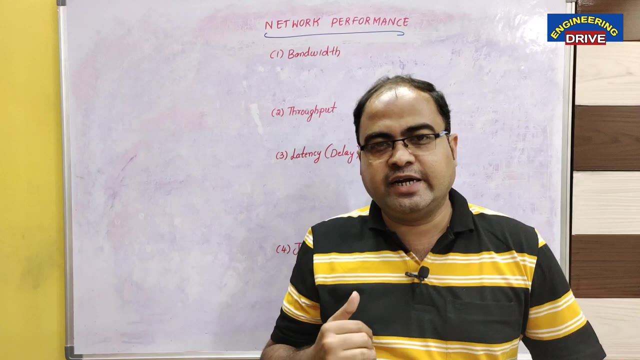 How much One liter water bottle is there with me Now? based on size of the water bottle, I can say it is bandwidth. What is the bandwidth of this water bottle? One liter water. Can I store more than one liter? It is not possible. Yes, of course I can store less than one. 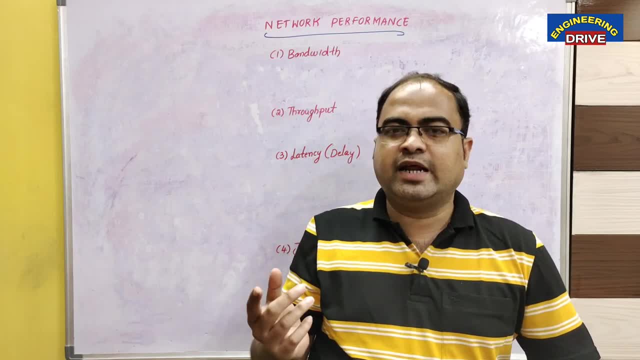 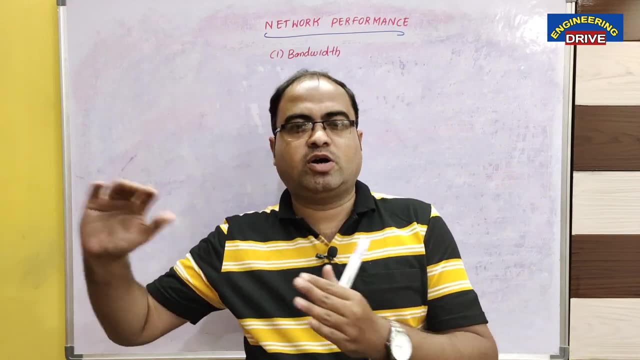 liter, but more than one liter it is not possible. So what is the bandwidth of this water bottle? It is a water tank. From water tank. the water needs to flow to some other place or to some taps, and one inch pipe is there. Now, if we 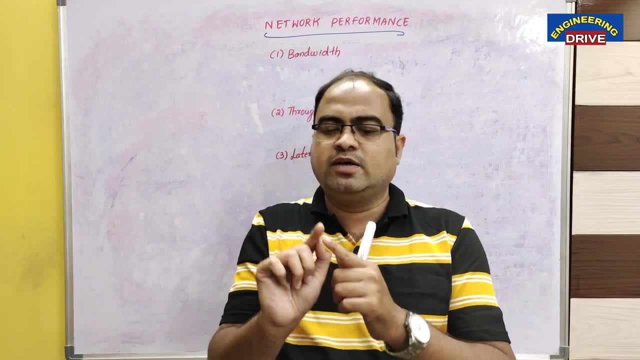 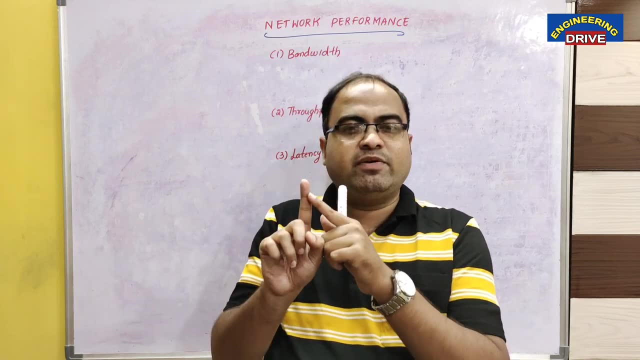 have the one inch pipe, then maximum the transmission of water can take place within that one inch capacity only. Beyond that it is not possible to transmit the data because the bandwidth of that pipe is one inch only. Similarly, here also in networking terminology, bandwidth. 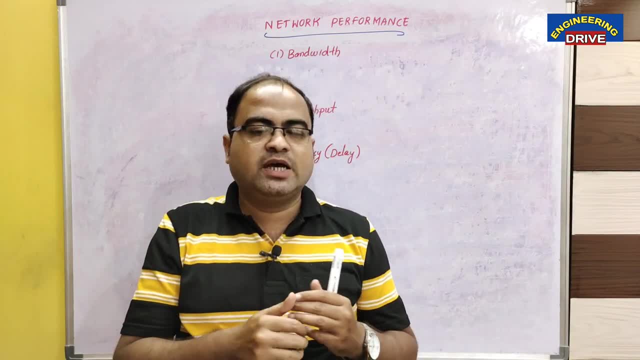 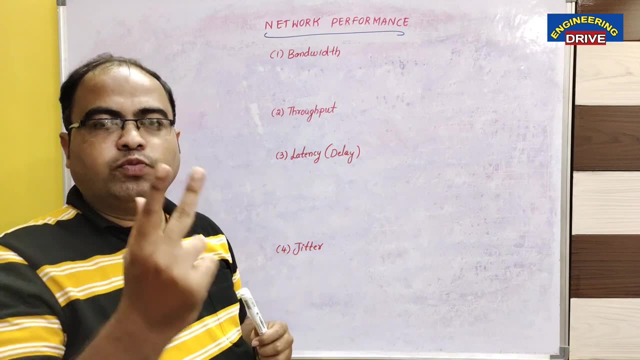 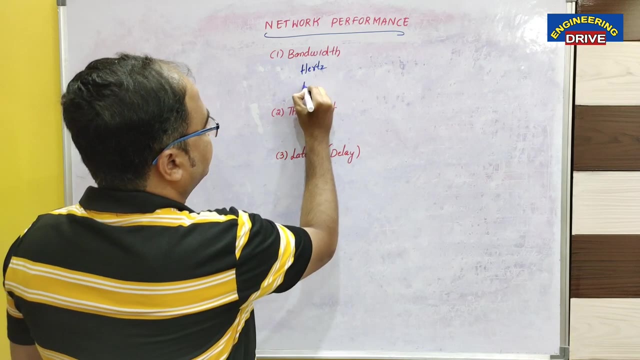 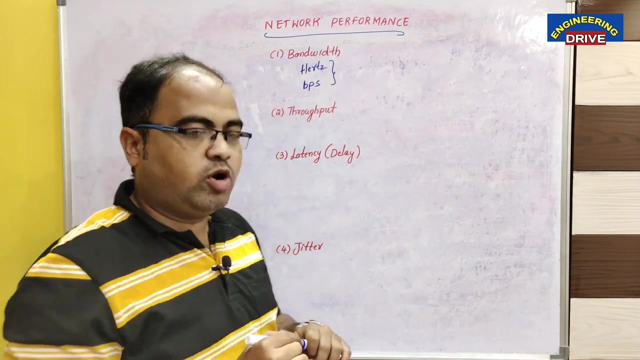 is nothing, but There is literally a minimum capacity by which the data can be transmitted. That is a bandwidth. Now, this bandwidth, it can be measured in two ways: One is in Hertz, Another one is in bits per second. So these are the two ways in which we can measure the bandwidth. 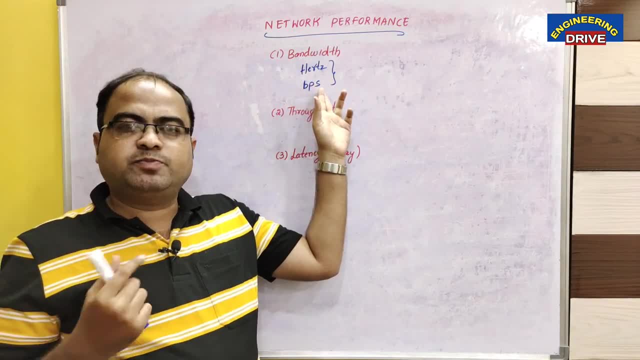 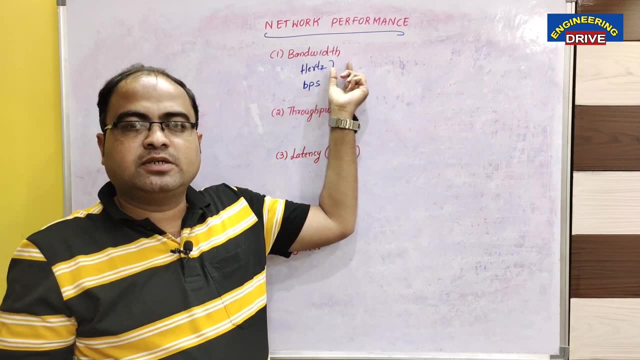 of a network. One is Hertz, another one is bits per second. Sir, when we need to measure in Hertz and when we need to measure inAdvertiseCT? Hello, bits per second, when we are measuring the frequencies that have been transmitted. that. 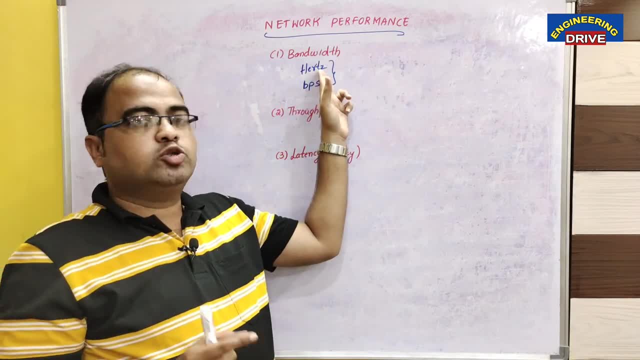 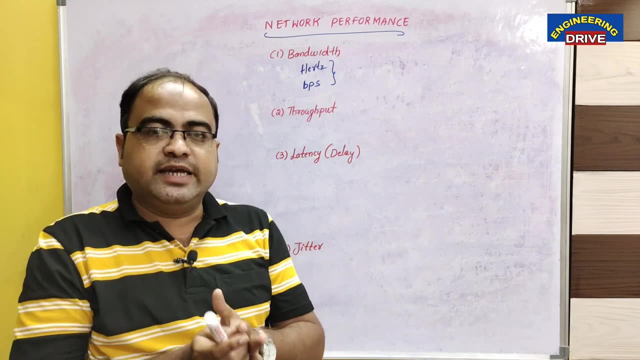 have been transmitted in a network, then at that time we need to make use of hertz in order to measure the bandwidth. When the data is transmitted in a normal manner, other than frequencies, then it needs to be measured in bits per second. So these are the two important differences. 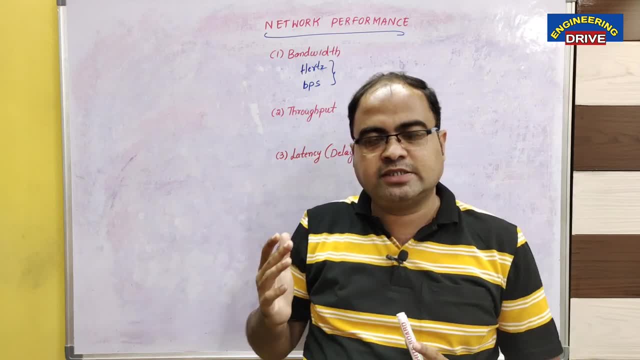 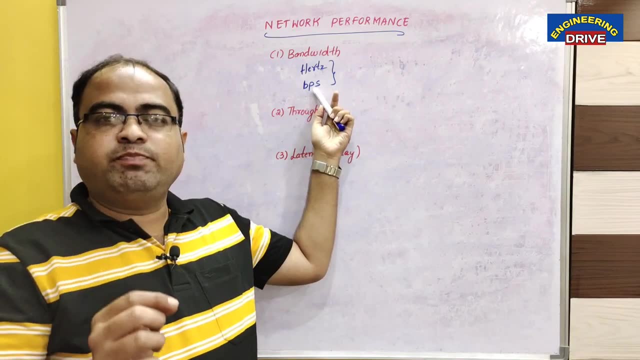 So when we are measuring the frequencies, makes use of hertz, and when we are talking about the data- how much data has been transmitted in a network- then it is better to make use of bits per second. So these are the two ways in which we can measure the bandwidth of a network. 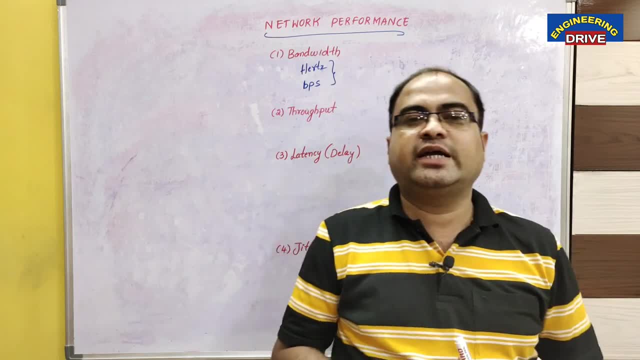 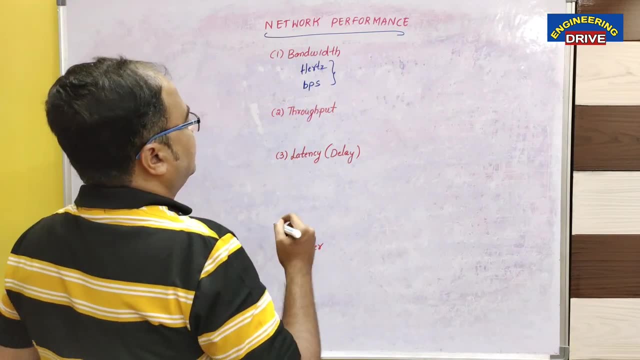 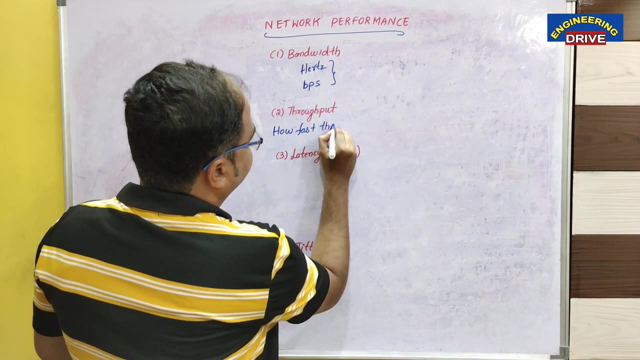 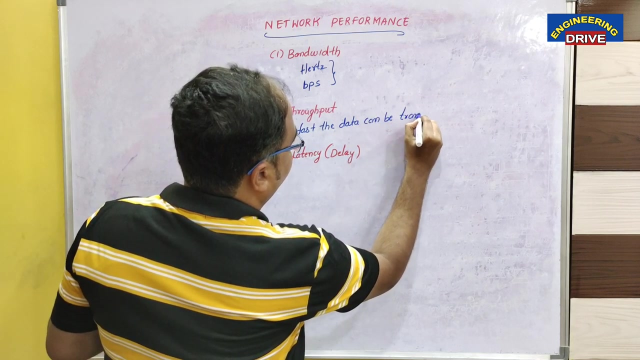 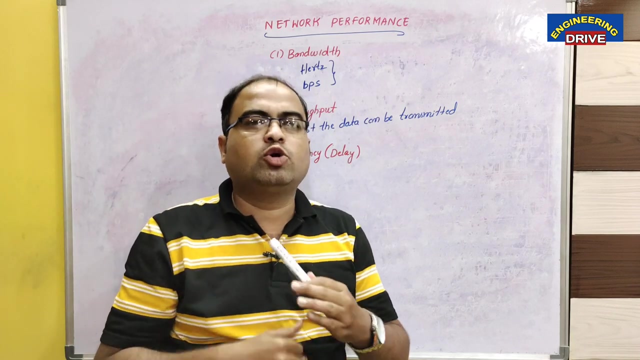 And while coming to the second way in which we can judge the performance of a network is a throughput. You know what is the meaning of throughput. Throughput is nothing but how fast the network, how fast the data can be transmitted. Now you only tell me throughput should be more or throughput should be less, if you want. 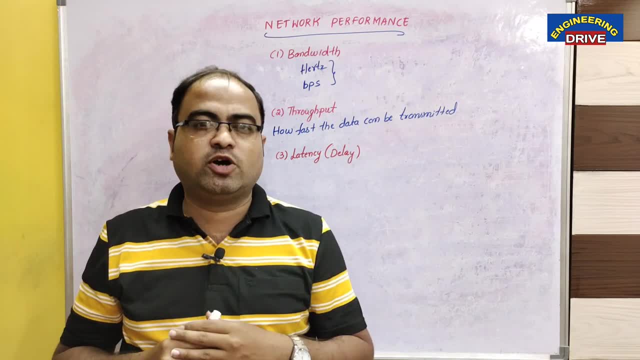 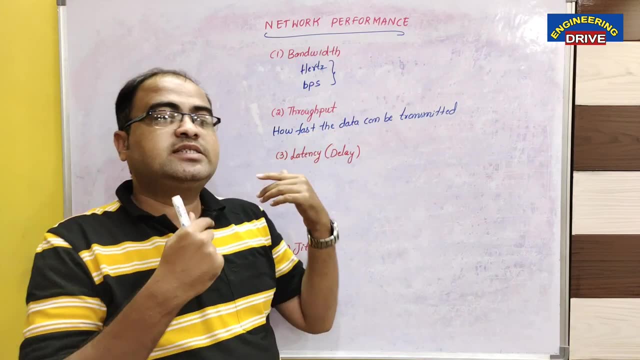 to improve the quality of our network. if you want to improve the speed of the network, compulsory throughput should be more, Because if the what is throughput- It says that how fast the data can be transmitted, it is nothing but the throughput. 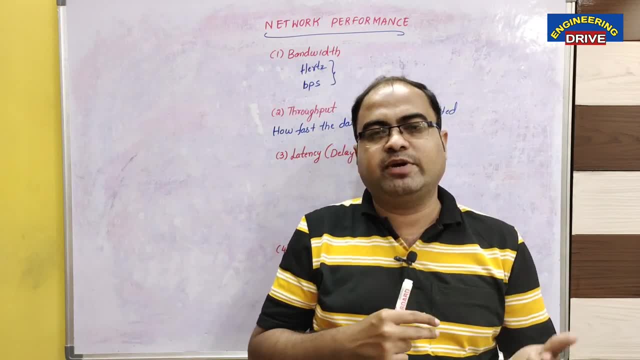 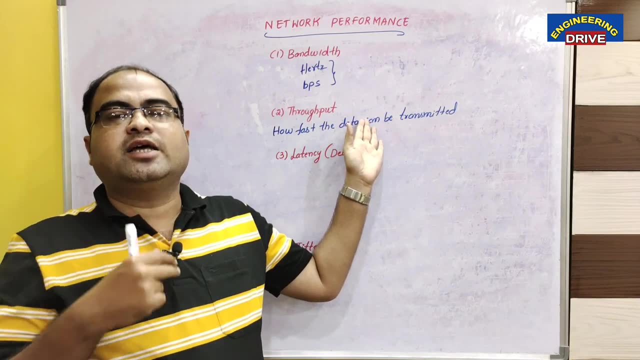 So if the throughput is more, Then more amount of data can be transmitted to the devices in the network. This is the second way. If the throughput of the network is more, then the performance of the network is good. So based on throughput, the network performance can be determined. 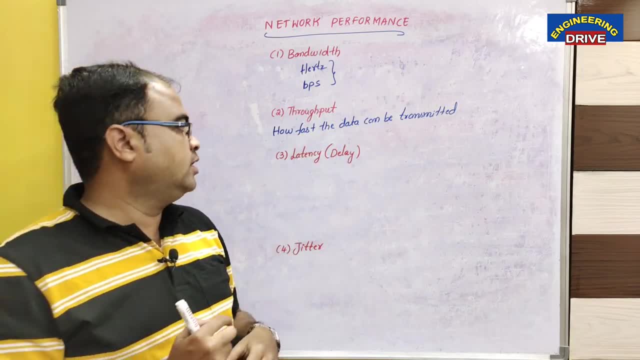 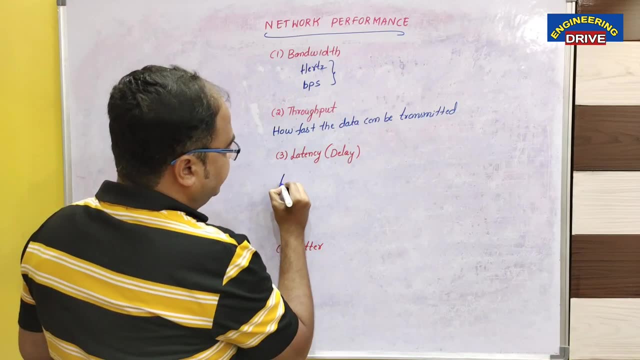 This is the second parameter, And while coming to the third one, that is, latency, You know what is the meaning of latency, or what is the meaning of delay? Dear students, let us say: from device A to device B, one message is ready. 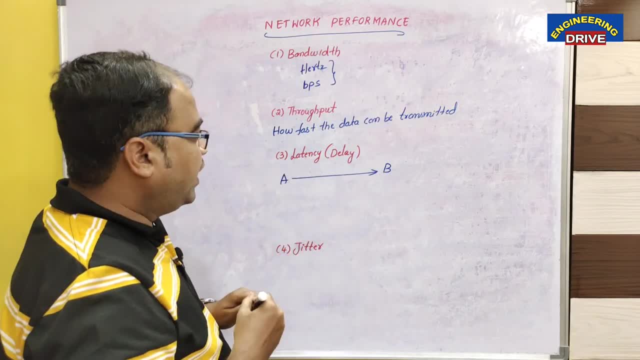 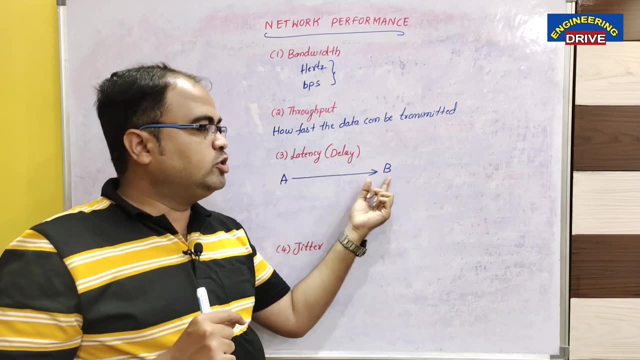 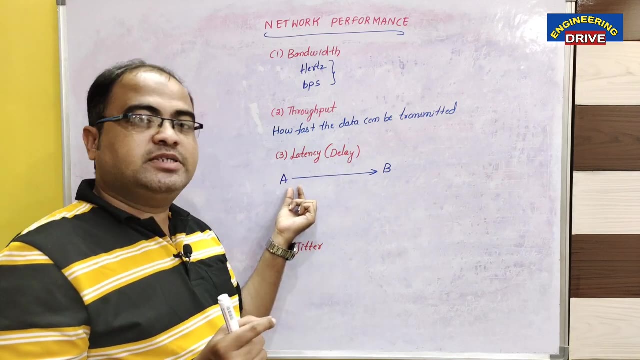 In At device A. I want to transmit to device B. Now, what is latency? Latency says that how long it will take for the entire message to be received by B. What is latency? It says that how much amount of time it takes for the message to receive to the destination. 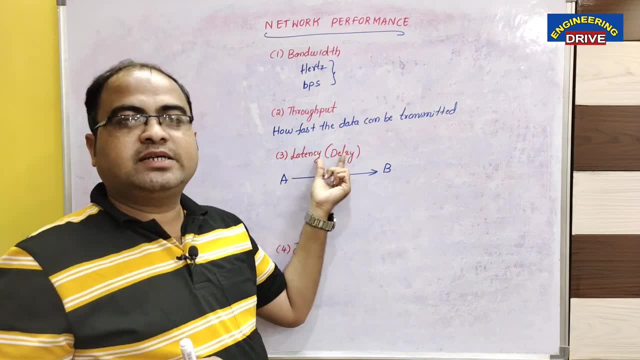 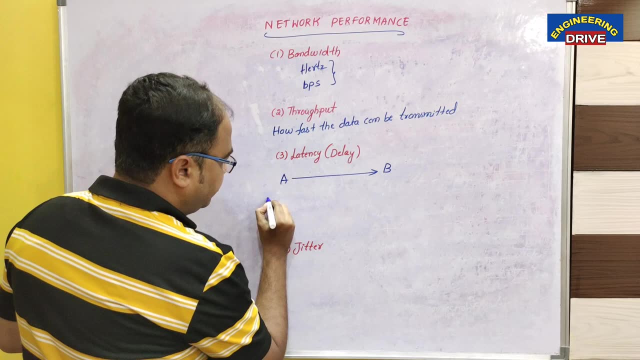 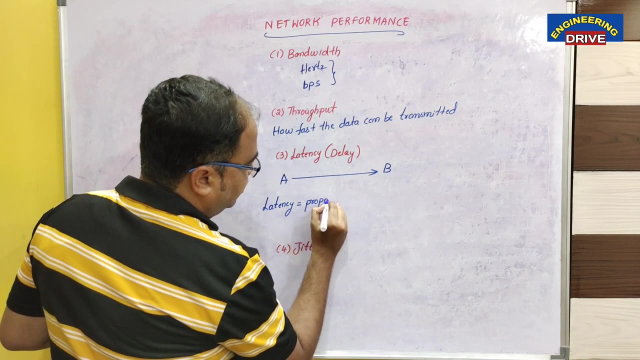 Where is the destination? At B. So that entire time is nothing but the latency or delay. And in order to measure this latency, there is one formula, Accurate formula. The latency can be measured by using: latency is equal to propagation time. 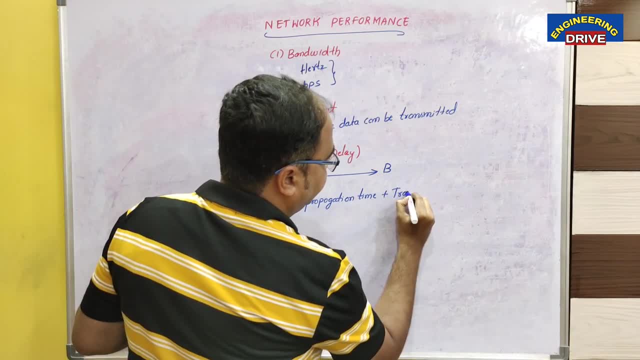 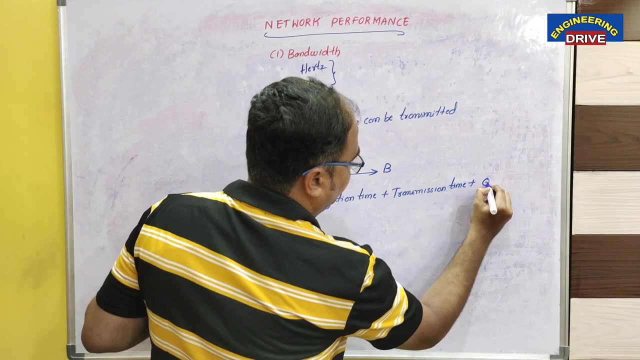 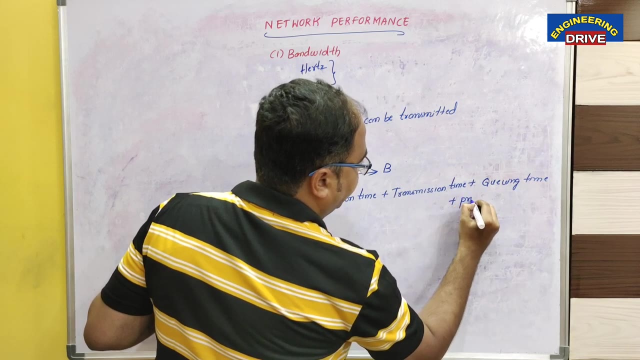 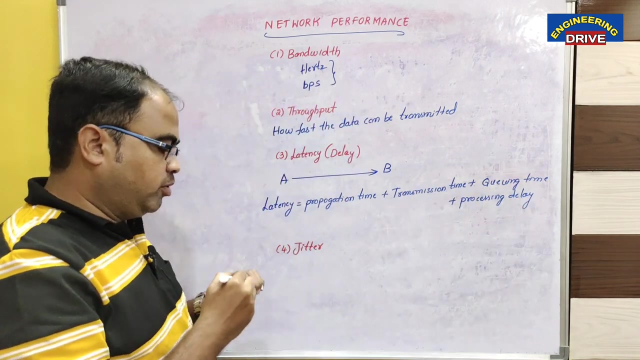 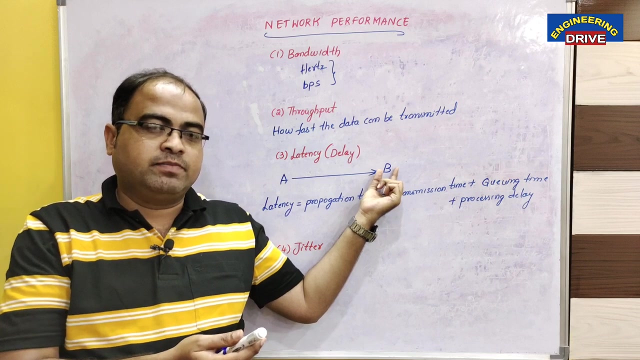 Plus transmission time, Plus queuing time And Plus processing Delay. So this is the accurate formula. Okay, Just now I told that how long the entire message will take to reach to B is a latency, But the accurate definition of latency is this one: 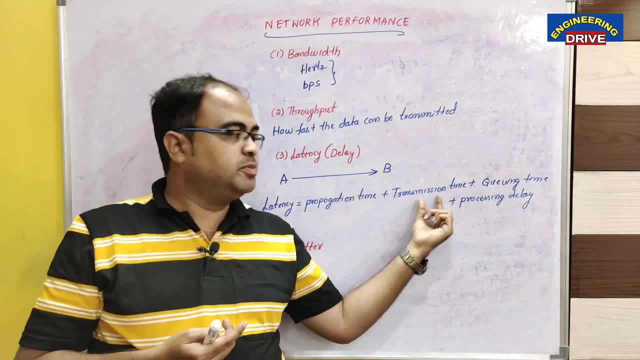 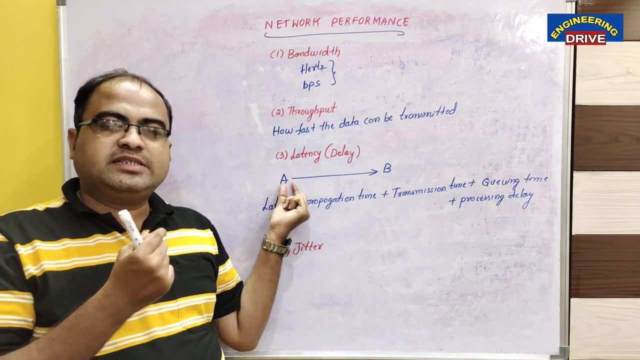 It is a combination of these four: Propagation time, Transmission time, Queuing time And processing delay. What is the meaning of propagation time? Propagation time is nothing but when the message has been sent from A to B And From A. 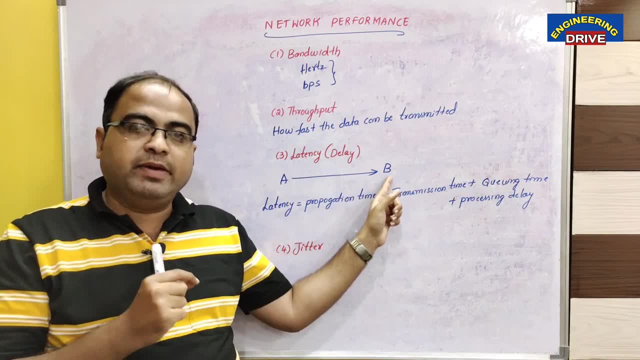 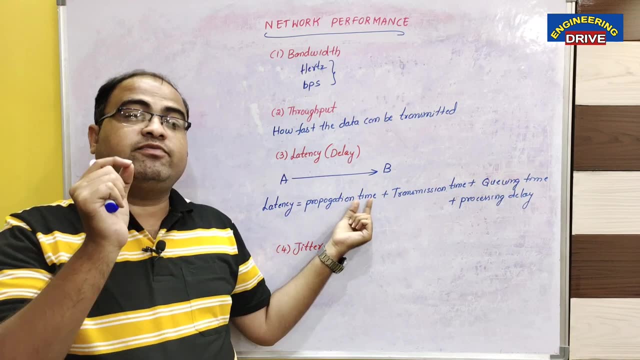 To B. When the first bit of the message will reach to B, Then that time is nothing but the propagation time. Here I am not saying the entire message should reach to B. I am saying that whenever the first bit of message Will be delivered to B. 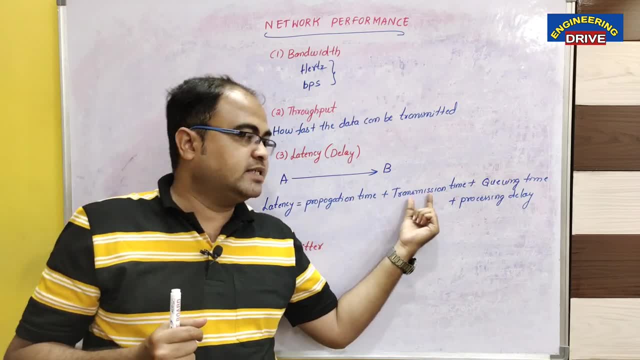 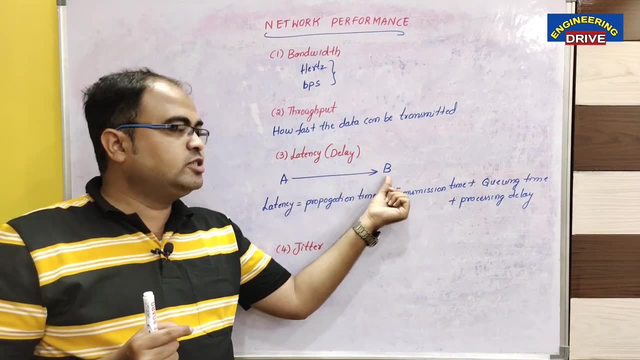 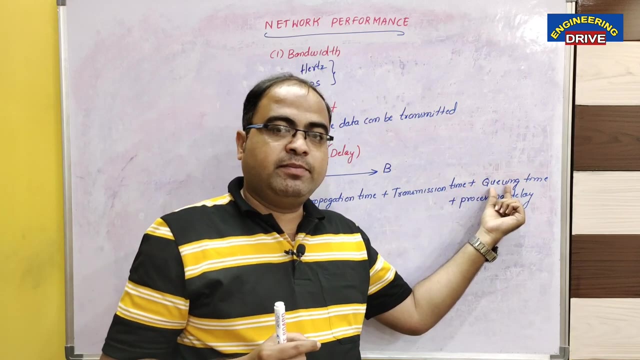 That is nothing but the propagation time. And then the second parameter: Transmission time. Transmission time is nothing but the time that has taken For the entire message to reach to B. The entire time is nothing but the transmission time. Okay, now, what is queuing time here? Queuing time is nothing but in order to reach the message from. 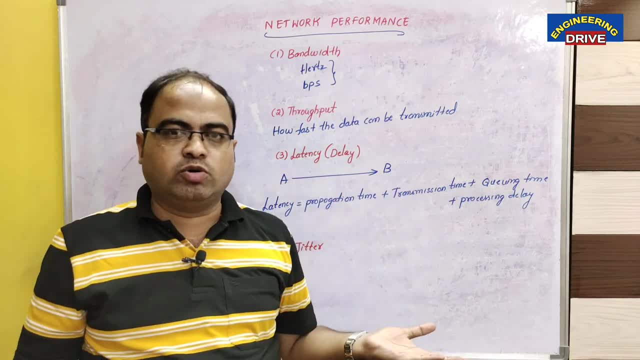 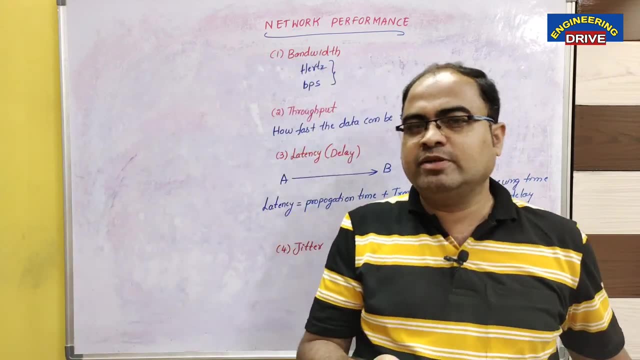 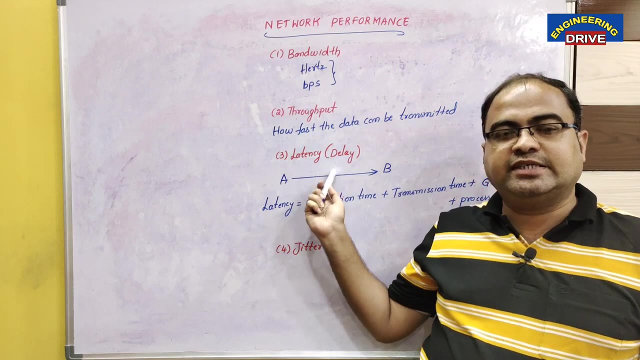 A to B. there are several devices in between them. we do not know, because in network not only two devices are available, but in between multiple devices are available. Queuing time is nothing, but in order to reach the message from A to B, there will be some mediator devices. there will be some. 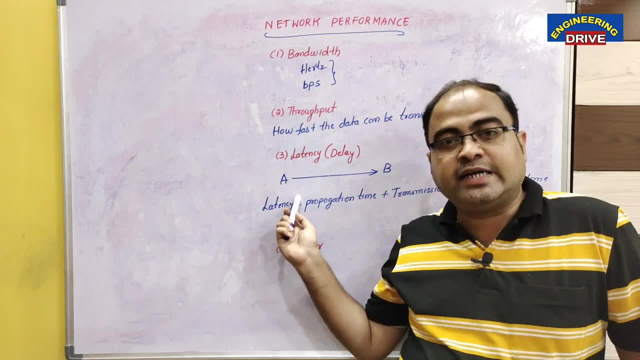 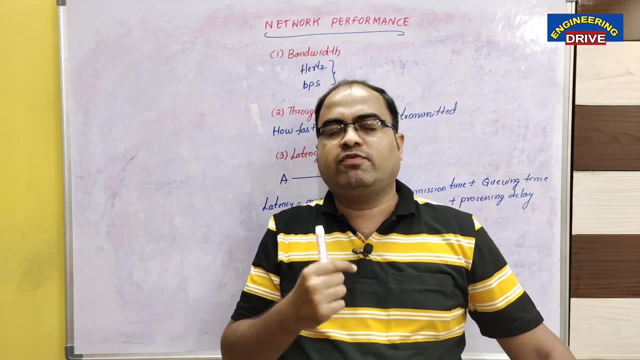 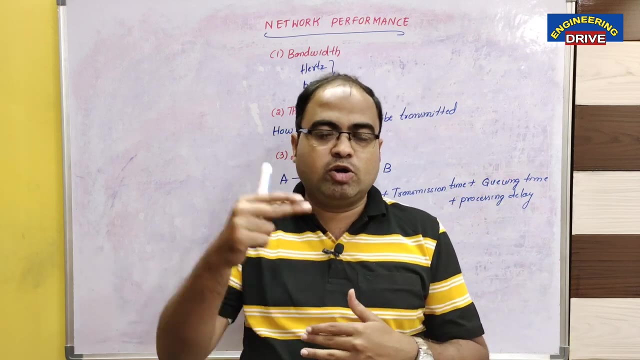 other networking devices. So how long the message will wait at that devices? that is nothing but queuing time. Best example: real time example. I will tell you: if I want to go from one city to another city, there will be several tall gates most probably we may get, depending on the kilometer. 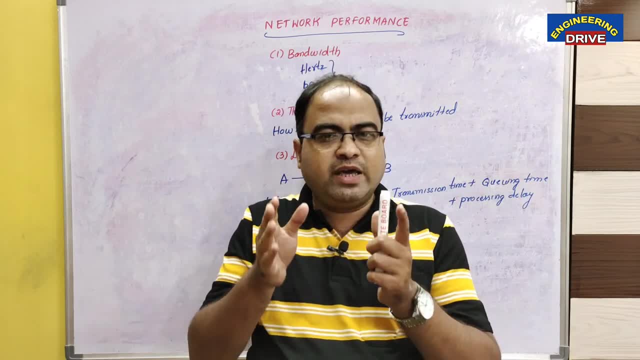 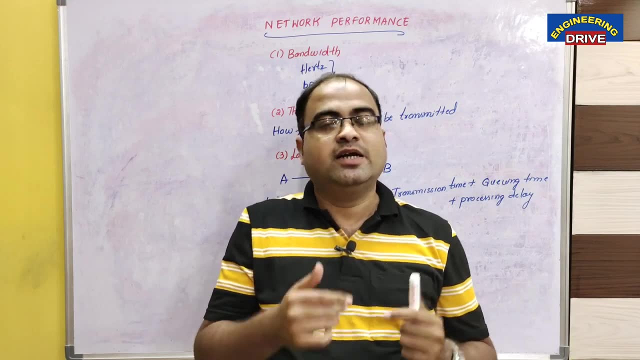 distance we may get two to three tall gates, is it right? So whenever a tall gate will come, what we need to do, I need to wait there. that will become my queuing time, is it right? Same here: the net, those networking devices at. at those networking devices, the message should wait for. 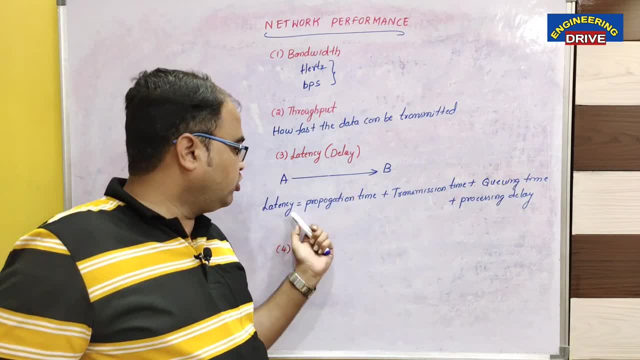 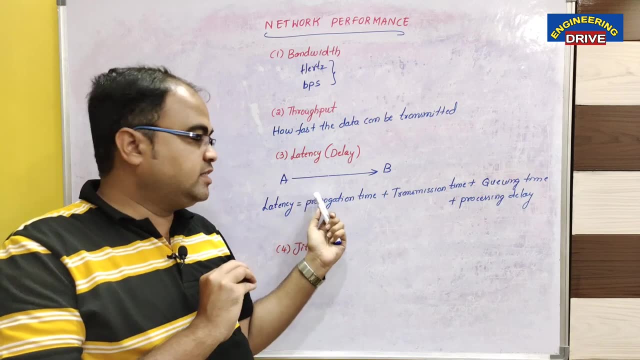 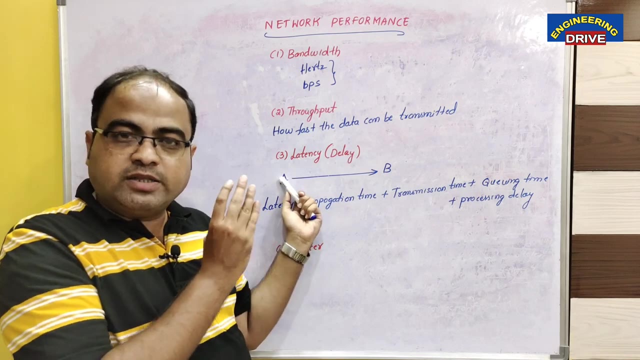 some time. that time is nothing but queuing time, and the last parameter to find out the latency is the processing delay. So what is processing delay? How long it will take for the message to sent from A, because at A the message need to be. processing should be performed. 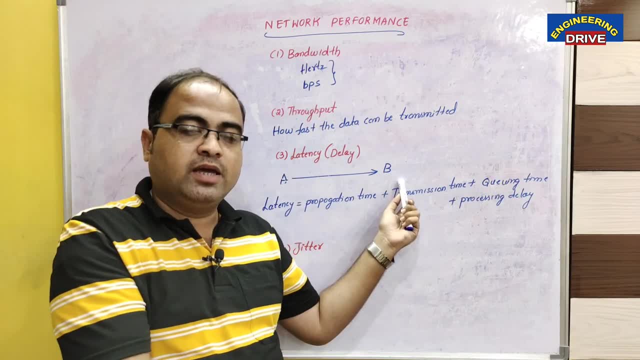 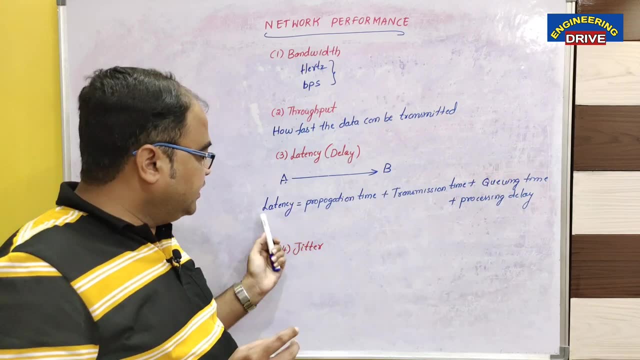 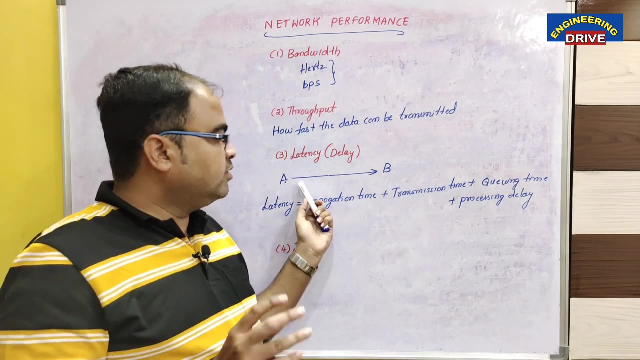 on that particular message at A. Similarly, once the message is resue to B, at B side, processing done, so that time is nothing but the processing delay. so, dear students, when we add all these values, then we will get the latency. so latency doesn't mean that some people will get. 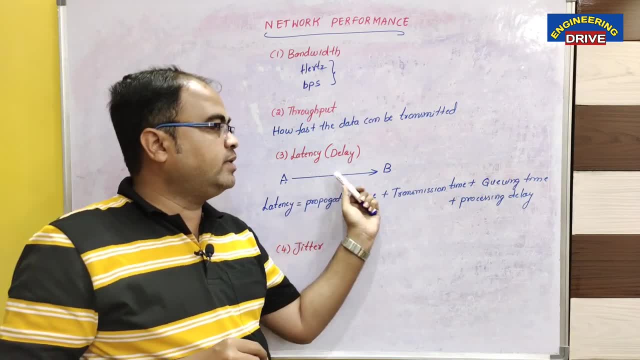 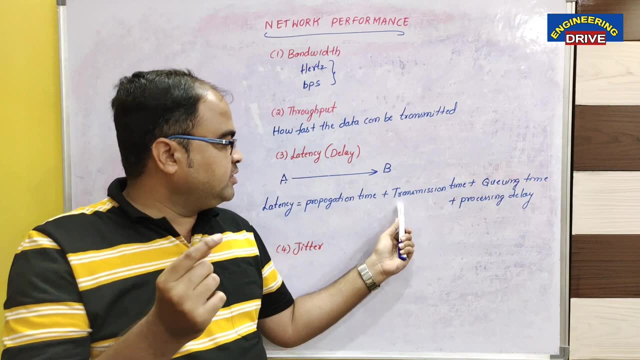 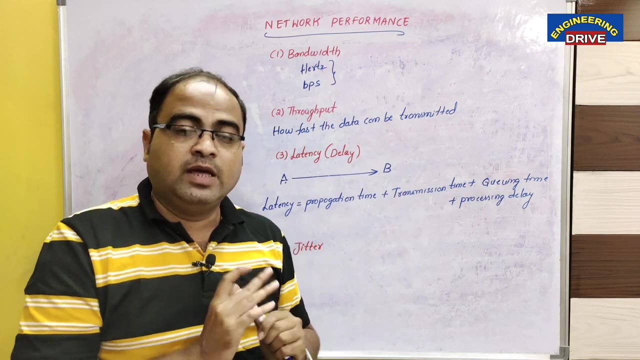 confused, sir. you told that latency is nothing but the entire time taken to reach to b. that is transmission time. no, sir, yes, but there is a small difference. transmission time is how the time that has been taken for the message to reach from a to b is transmission time. here i am saying the. 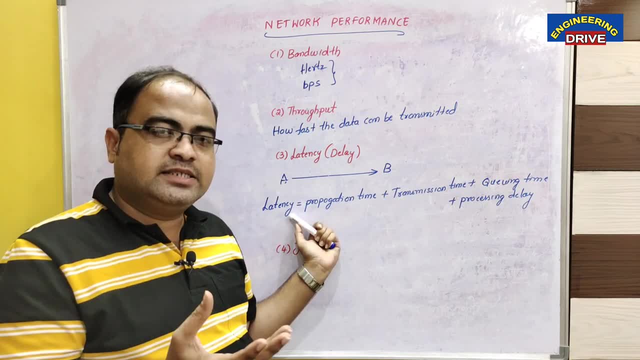 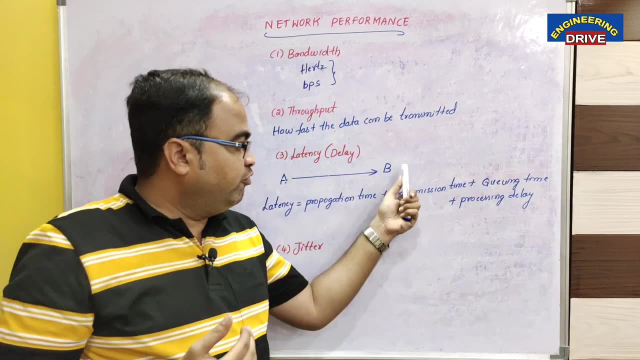 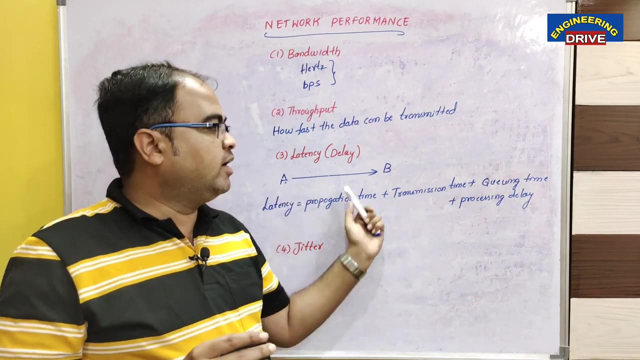 slightly different way. translatancy latency. i am saying that how long we will take to retake the entire message, to receive the entire message. when will we receive the entire message? you know when all these things should be completed: propagation time should be completed, transmission time should be completed, queuing time should be completed. processing delay should be completed. 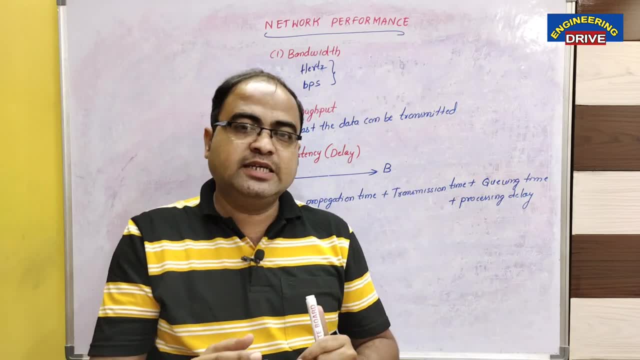 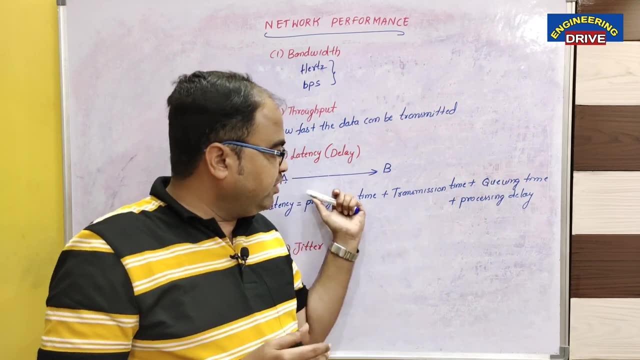 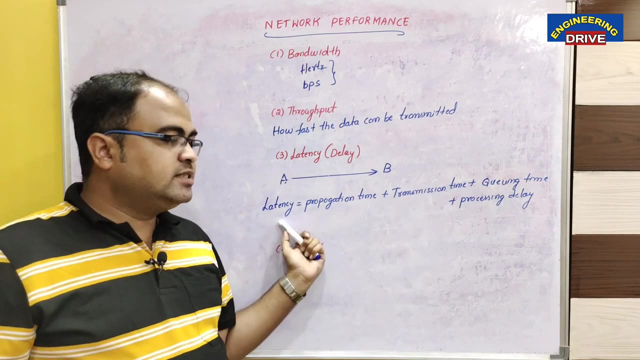 then we will receive the complete message. This is known as latency In way of explanation. in English. it may look similar, But when you use this formula, then you will come to know the difference between a latency and a transmission time. So in latency, delay will occur Because of this also. it will affect the network performance. Now, if I ask you latency should be minimum or maximum to improve the network performance, The answer is: latency should be minimum. delay should be minimum to improve the network performance. Is it okay? And the last way? 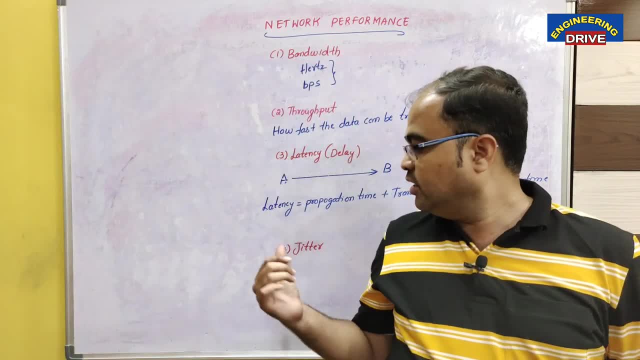 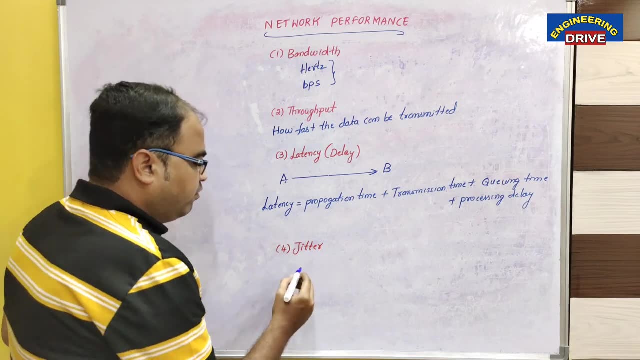 the last parameter based on which we can judge the performance is a jitter. Okay, what is actually a jitter here, Dear students? jitter is nothing, but when different packets have been sent from A to B. you know that messages are transmitted in the form of packets. Now, 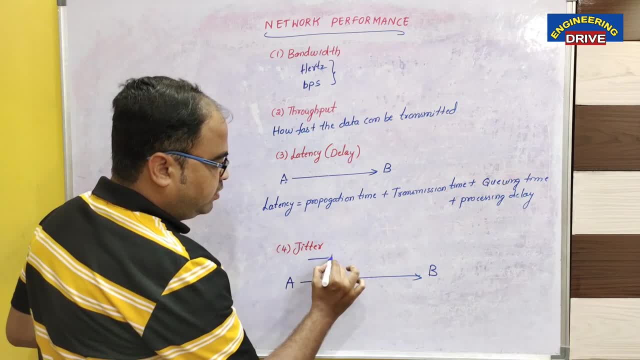 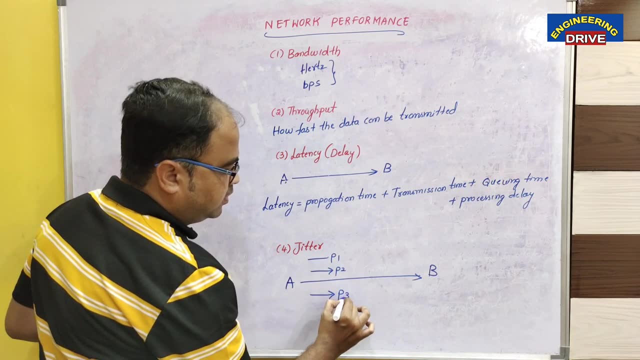 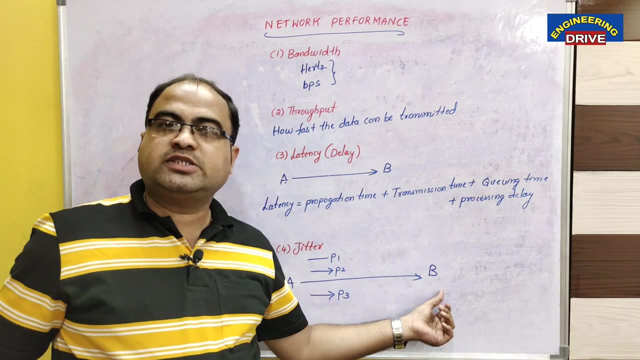 let us say three different packets: packet 1 and packet 2, and here packet 3.. Three packets have been sent to the receiver B. Now, for all these three packets, only two packets have been sent to B. Remaining third packet got delayed. Okay, why third packet got delayed? Due to some traffic. 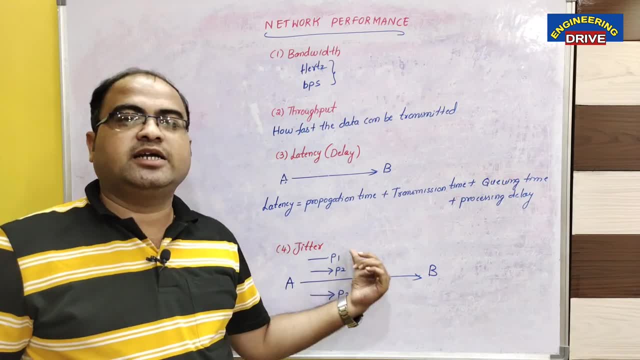 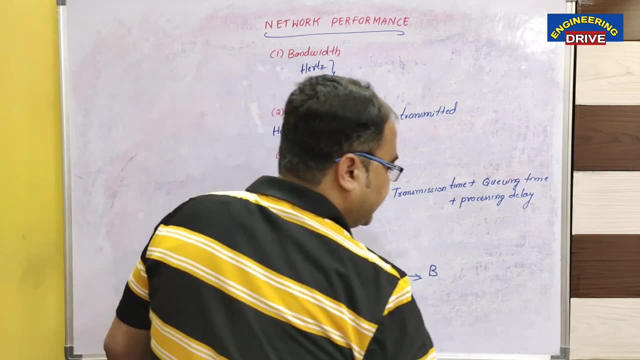 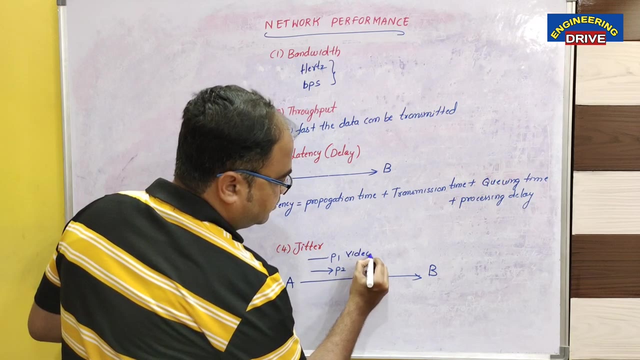 problem. Then at that time, what happened? We can say that jitter is there in the network, Is it right? I will give one more example. Instead of these three packets, let us take, there are two packets which has to be transmitted to B. Packet 1 contains video signals and packet 2 contains audio signals.